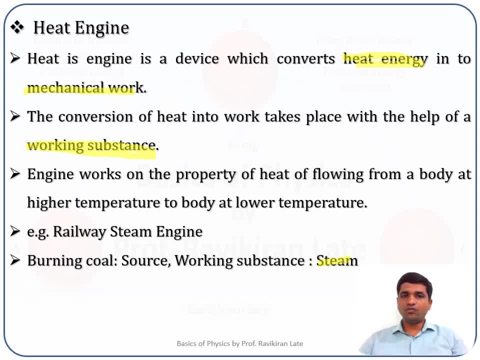 working substance and we know that heat flows from a hot body or body at a higher temperature to body at a lower temperature. in this way, heat flows according to the second law of thermodynamics. it happens naturally so that phenomenon is utilized in case of an engine. so first engine which was there. 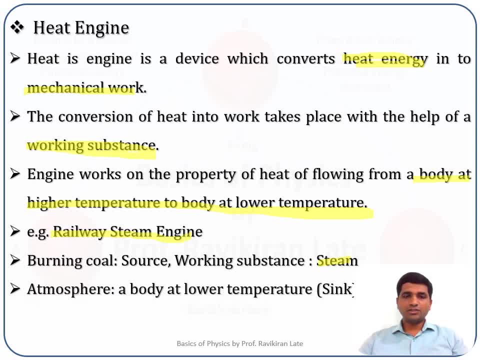 for example, it is a steam engine. in case of a steam engine source of heat, it is nothing but the burning coal is referred as a source of heat which is at a higher temperature, and steam which is prepared with the help of this source. it is considered as an working substance. 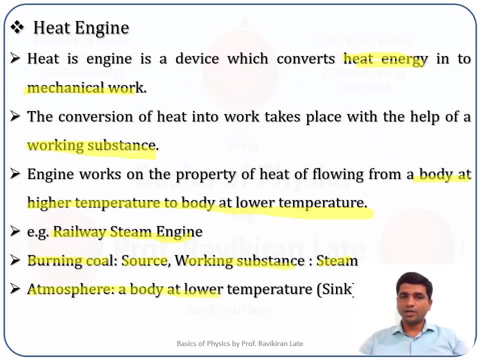 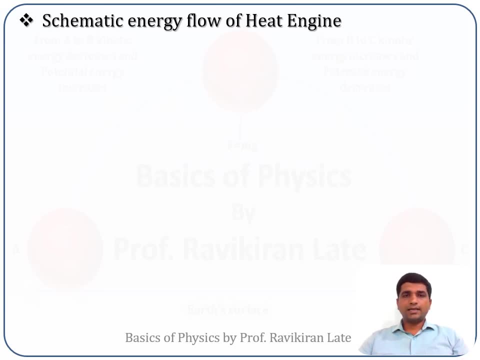 and this atmosphere, which is at a lower temperature as compared to the source, which is a burning coal. that is nothing but the sink in this case. okay, so in case of a steam engine, now we will discuss a schematic energy flow of a any heat engine. we know that, naturally, heat can flow. 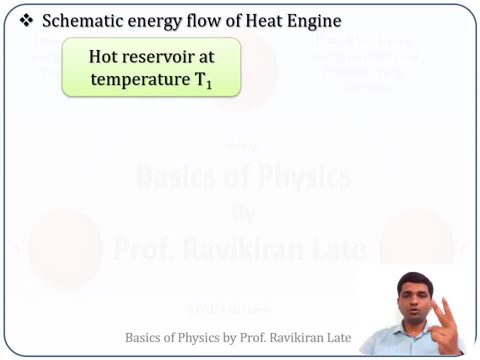 from higher temperature to a lower temperature. so basically, two parts are there in any design of an engine. the one is the heat reservoir, which is at the temperature T 1, which is relatively high temperature, and the reservoir which a cold to the reservoir. it is at a temperature center or medium temperature. 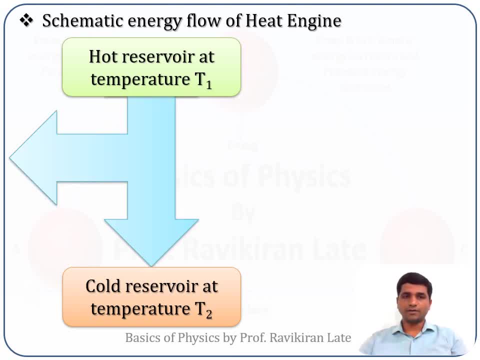 temperature, T2, or which is at a relatively lower temperature. okay now, when heat flows from hot region to the cold region, when heat flows from source to the sink or hot region to the cold region, we can convert some part of this heat into the energy so device which is used for this purpose. 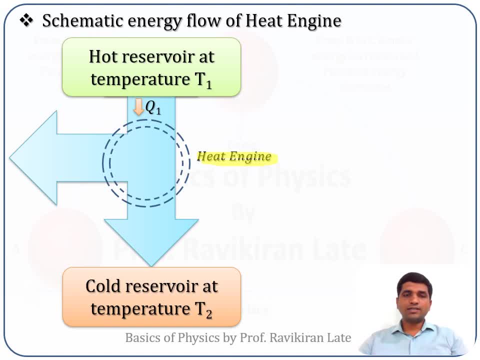 that we call it as a heat engine. okay, so let us say that Q1 is the amount of heat which is given, taken from the hot reservoir, and let us say Q2 amount of heat it is given to the sink which is at a lower temperature. so the net amount of heat, which will be Q1 minus Q2, it will be converted. 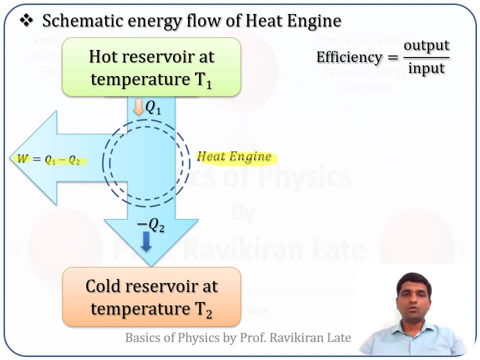 into the work. it will be converted into the work. so we are getting some amount of work done. now, how you decide the quality of that heat engine? it is the parameter which we call it as an efficiency, which is nothing but the output work we are getting to the input energy which is provided. so efficiency can be defined in the form: 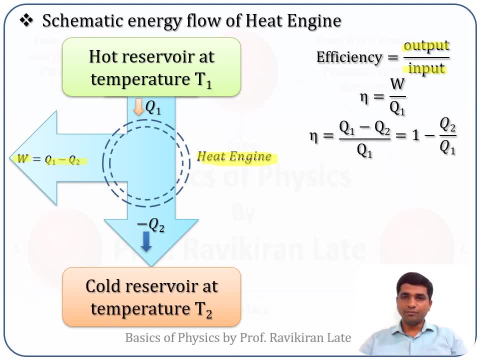 work obtained to the amount of heat given to the system. but we know that initially in this case we had given the Q1 amount of heat and this Q2 amount of heat is it was rejected to the sink. okay, so net amount of heat which is converted into the work, it is nothing but the Q1 amount of heat which is. 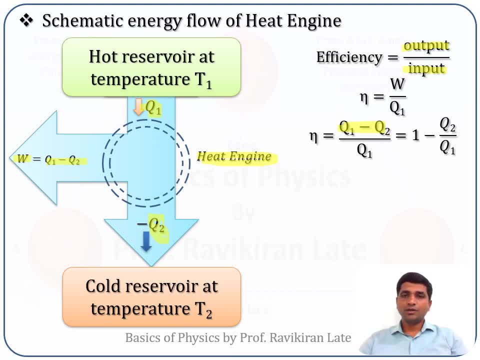 given to the heat which is given to the system. so we have to calculate the efficiency of the heat which is given to the system. so we are taking the Q1 minus Q2, so W we can substitute as a Q1 minus Q2 divided by Q1, so you get 1 minus Q2 by Q1. that is an efficiency of a, any engine. you can calculate by. 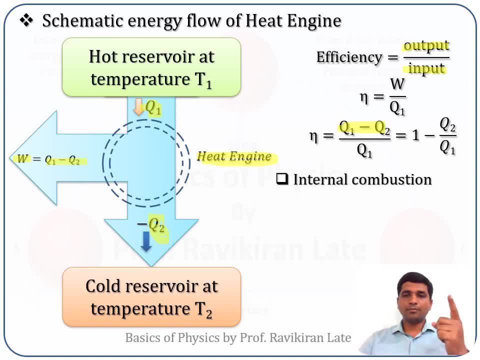 this formula. basically, there are two types of engines are there? what are those two types of engines? the first one is the internal combustion engine and second one is that is called as a. These are nothing but the petrol engine, which we call it as an auto engine, and the diesel engine. These types of engines, they are nowadays used majorly. But in addition to that, one external combustion type of engine is there, which is nothing but a steam engine. 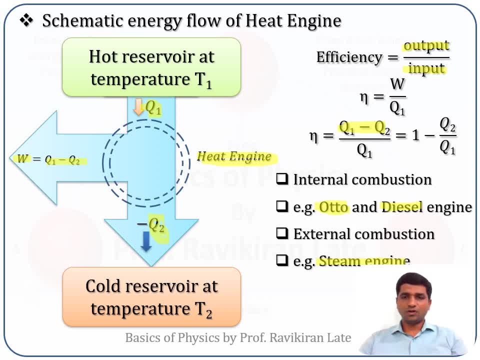 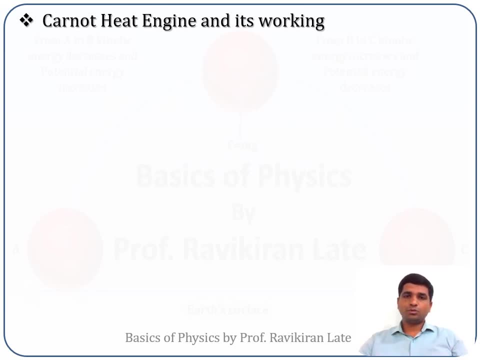 Nowadays no one uses steam engine for this purpose. So in our syllabus now, in our topic of this presentation, we will be discussing now auto engine and diesel engine in the detail. But prior to going to the auto engine or a diesel engine, let me show you the first theoretical engine, which was proposed by a French physicist, Carnot, in the 18th century. 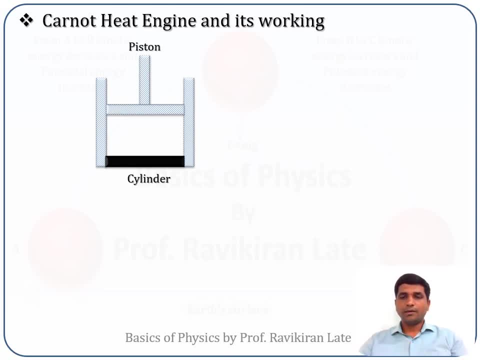 18th century. that is nothing but the Carnot heat engine. It was a theoretical engine which was proposed by this French physicist. It consists of a cylinder fitted with a piston which can move freely without a friction through this surface. And if you consider this cylinder, the sides of these cylinders, these are made up of insulating material. 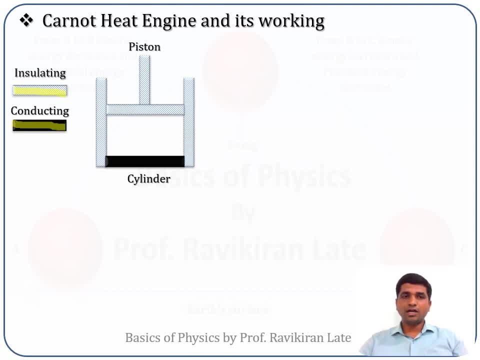 And the base of this cylinder is made up of insulating material And the base of this cylinder is made up of a conducting material. So this is the cylinder which is the main part of this Carnot heat engine. Next part, it is the source which is at a temperature T1.. 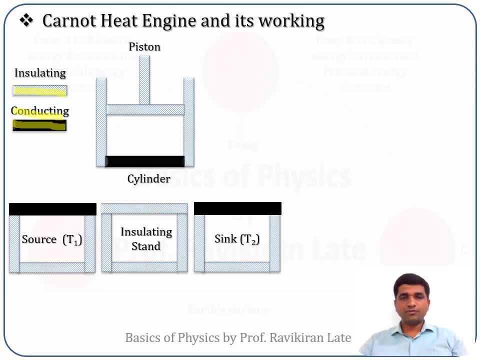 Insulating stand is there and sink is there, which is maintained at a lower temperature- T2- as compared to the source. Now, if you consider a reversible Carnot cycle, it consists of four operations. What are those four operations? The first operation: it is an isothermal expansion in which this sink, it is placed on the source. 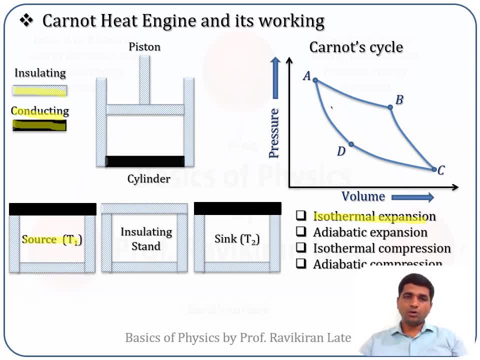 It is placed on the source, so as the lower surface of this cylinder and the upper surface of this source. they are both conducting in nature. So the amount of heat will be given by this source to this gas molecules which has enclosed within this cylinder, and the gas will expand isothermally. 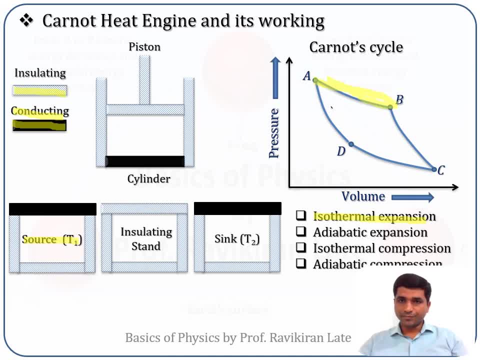 So it is shown with the curve AB in this diagram. It is shown with the curve AB in this diagram. Now, second operation: it is there that is adiabatic expansion. In that case the cylinder is moved from this source and it is placed on this insulating stand. 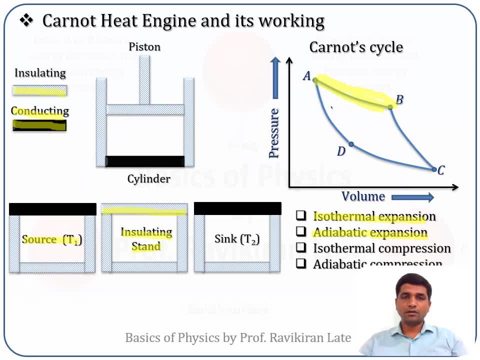 Now, if you consider the upper surface of this cylinder or this sink stand, it is insulating in nature. It is insulating in nature, so there will be no exchange of the heat with the gas molecules, molecules inside this cylinder. okay, so it is an adiabatic expansion, the curve it is shown. 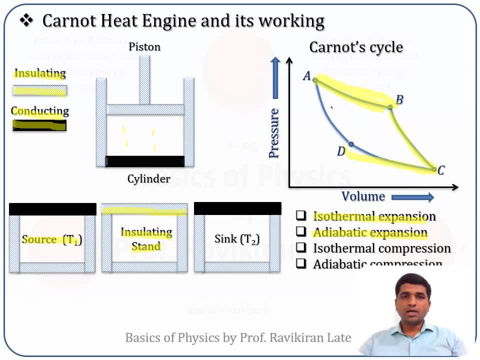 in this figure and the next time this cylinder. it is kept on this, this sink, which is at a relatively lower temperature and as these both are conducting in nature, the gas will gas which is enclosed inside this cylinder. it will give some amount of heat to this sink, so it will be an isothermal. 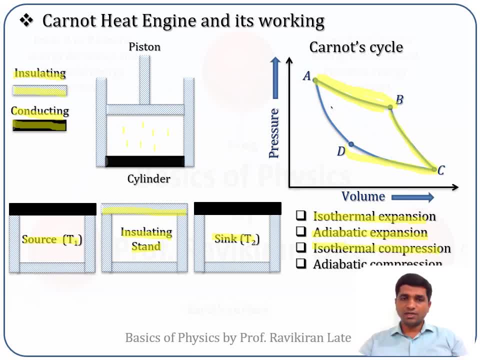 compression and in the last step, this cylinder. it will be removed from this sink and it will be kept on this insulating stand. so as insulating stand it does not take or give the any amount of heat with the cylinder. so it is an adiabatic compression, this kernold cycle. it has been 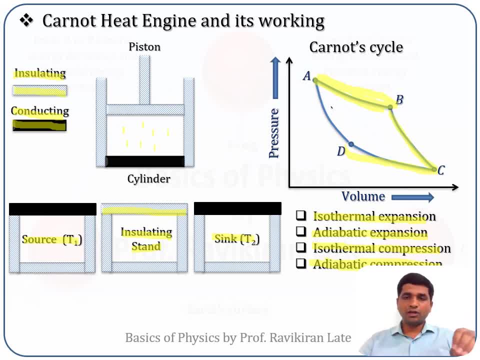 discussed in one of my previous lecture in detail. if you want, you can search kernold cycle in our playlist heat and thermodynamics. you will get a detailed description of this video. efficiency of the kernold cycle- it is given by n- is equal to t1 minus t2. divided by t1, t1 is the 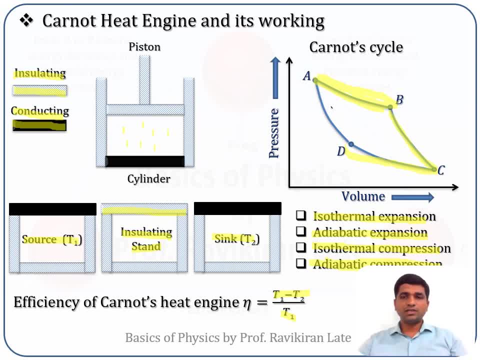 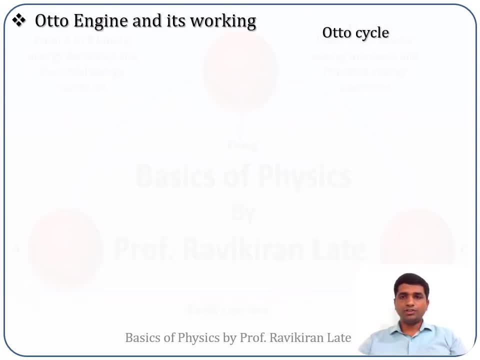 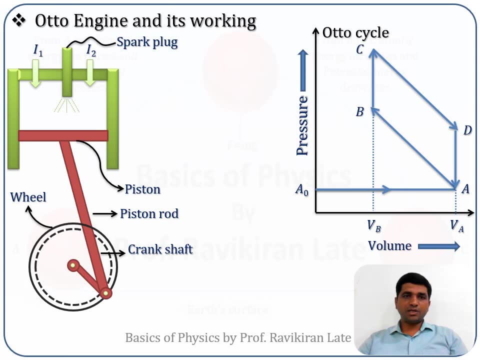 temperature of the source and t2 is the temperature of the sink. that's it for the kernold heat engine. now we will move ahead with the auto engine. now, what auto engine it is that we will discuss? auto engine consists of a piston fitted with a piston fitted under a cylinder, and the cylinder is that piston is connected with a wheel, with the 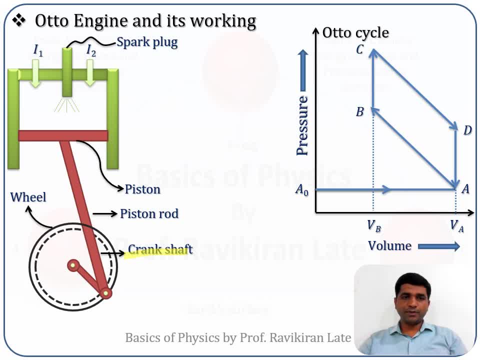 help of crank and shaft. okay, crank shaft arrangement is there and that is connected with a wheel and this, if you consider the cylinder which is fitted, in which the piston is fitted, there are two walls. are there i1 and i2? and spark plug, in which the piston is fitted. there are two walls. are? 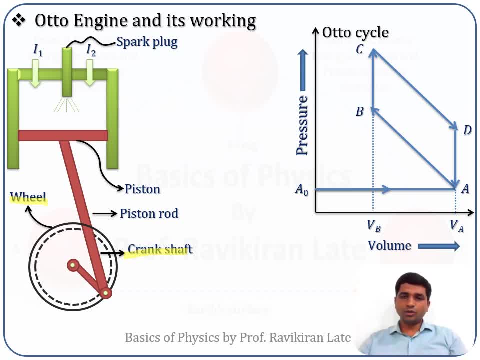 there, this auto engine which we are considering over here. these are nothing but the petrol engines which are discussing, we are using in our daily life. it, this auto engine. it has total six operations. these six operations are shown over here in this diagram. so these six operations are nothing but. 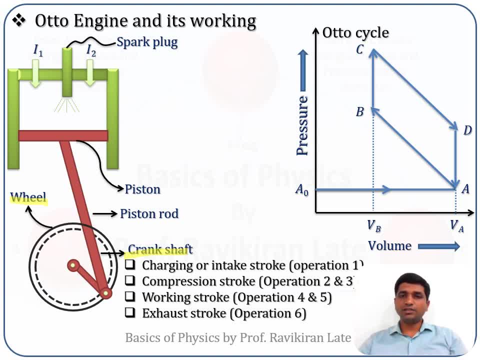 a naught to a, a to b, b to c, c to d, d to a and again, finally, a to a and again. finally, a to a and a. not these are the six operations. what are these six operations are there? we will be discussing in the detail in the next slides. prior to that one, let me tell you the efficiency of the auto engine. 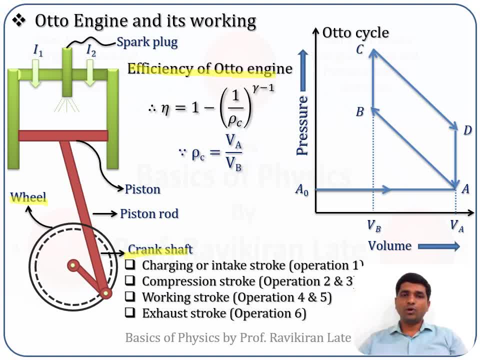 it is given by eta is equal to one minus one upon rho c, to the power gamma minus one. what is gamma? gamma is the. it is a compressibility ratio, uh, it's a ratio of specific heat at constant pressure to the specific heat at the constant volume and this rho c, that is the compressibility. 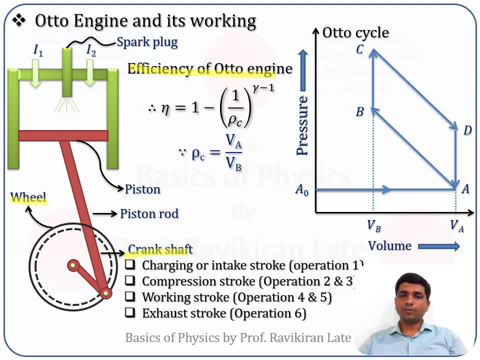 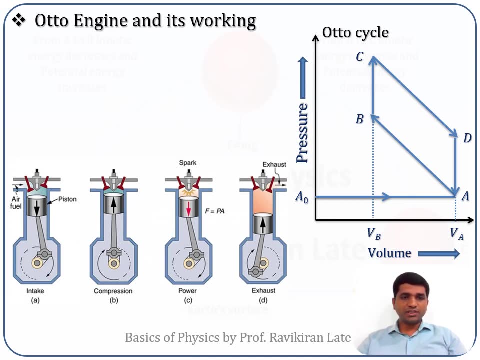 ratio, that is v a upon v b, that is the volume occupied by the gas molecules at the point a and the vb is the volume occupied at the point b. that is called as the compressibility ratio. now, if you consider, in this diagram i had shown, uh, the four different pictures are over, shown over. 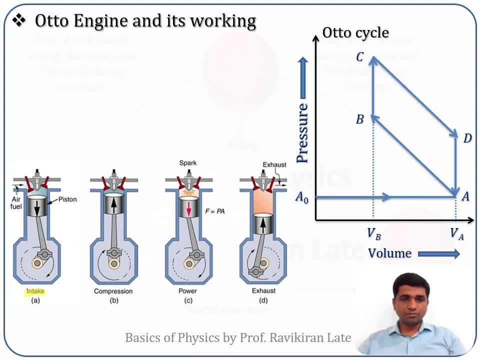 here. what are those four different pictures are suggesting us? first one is when the we are moving from the first part, that is, from a a naught to a, when we are moving from a naught to a, what happens? this is called as the charging stroke or intake stroke. 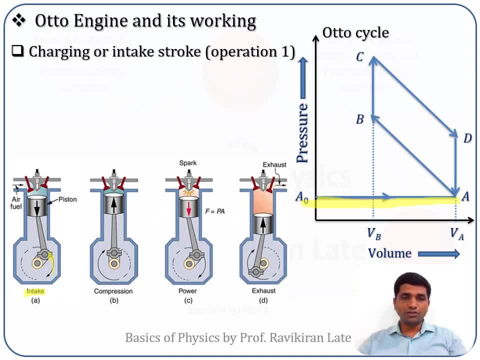 in which the wheel will rotate in this fashion from this point to this point and it will take fluid inside the chamber. it will take fluid or the working stroke substance which will be there. in case of an auto engine, it is a petrol plus air, two percent of. 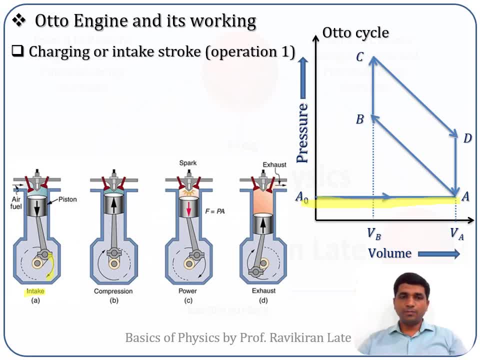 petrol and 98 percent of the uh air. it will be taken inside this cylinder- okay, it's the space between the piston and the spark plug- in the second operation, which consists of a operation, number two, and three, which consists of operation two and three, that is, from a to b and b to c. 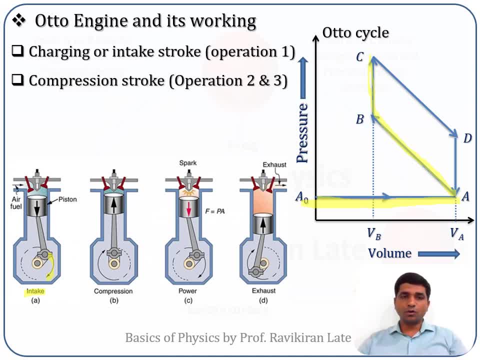 it is a compression stroke in which the wheel will rotate from this position to this position. as a result of that, this piston will move in the upward direction, this piston will move in upward direction, and as this piston will move in the upward direction, so that will be the compression. 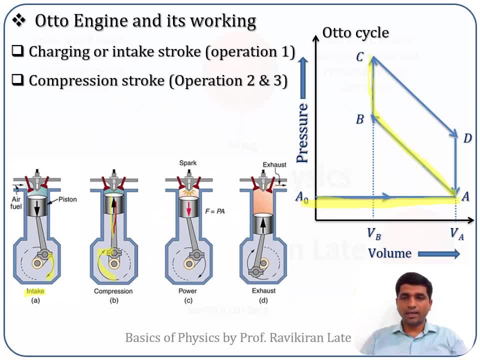 so, whatever the working substance- petrol and air- which is taken inside the chamber, it will be compressed. as a result of that, what happens? the temperature of the environment increases and the fuel ignite with the help of this spark plug. so in the third operation, which we call it as an working stroke or a power stroke, 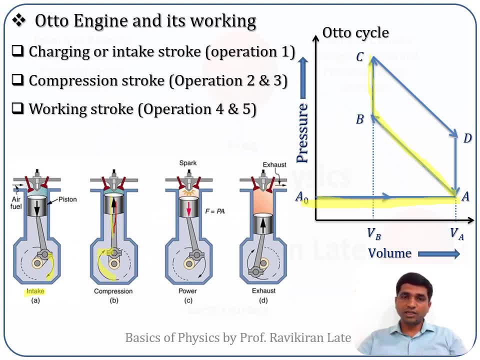 in this, the, due to the explosion inside this one, uh, the piston block, it will move in the downward direction, it will move in the downward direction and the pist as piston will move in the downward direction. so, due to that one, the volume will increase and that it is shown with the help. 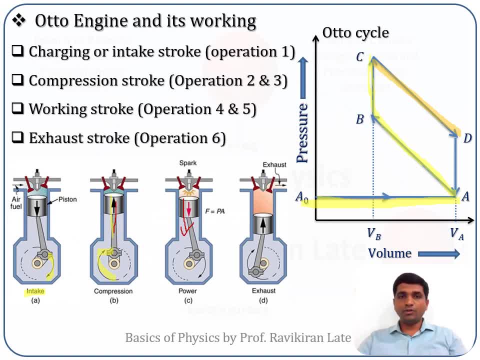 of this curve, a cd now in the last cycle. further its volume, it will be decreased. when this uh unused gases, or unused gases or unused fuel, it will be given to the sink. so this will happen at this point. so it is the amount of heat will be rejected during this process. so in case of an auto engine, it is the 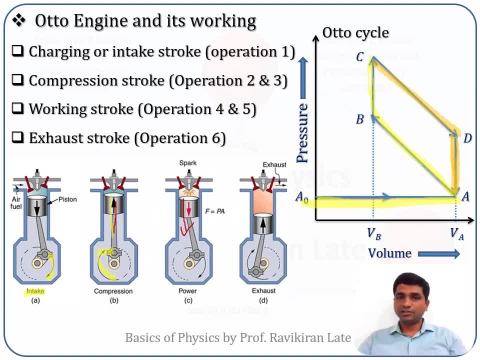 curve we see, during which heat is taken inside the system, and it is the curve during which the heat will be rejected to the sink and, in the final, from a to a naught, from a to a naught, which we call it as an exhaust stroke, the amount of there's a system, the cycle will regain its original. 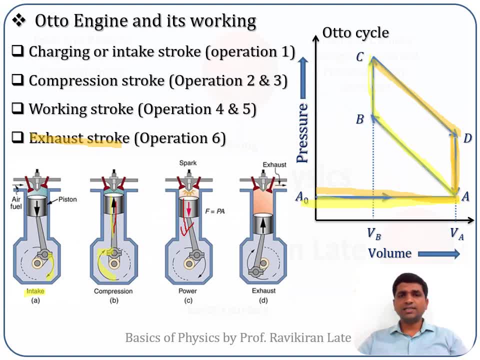 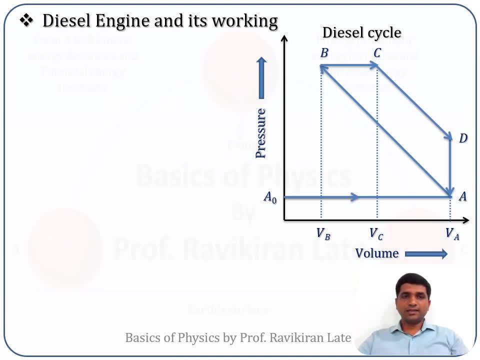 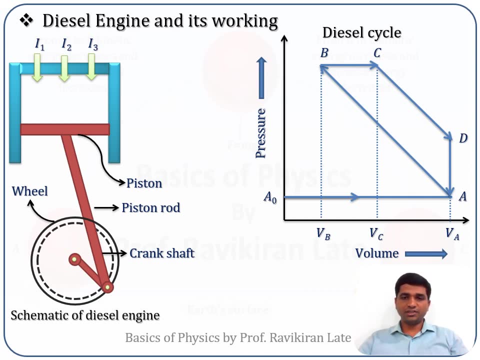 position and the cycle completes. these are the six operations which are involved in this auto engine. now next type of engine is there that is called as a diesel engine. what is diesel engine? diesel engine consists of the similar kind of arrangement which is there in the auto engine, just one. 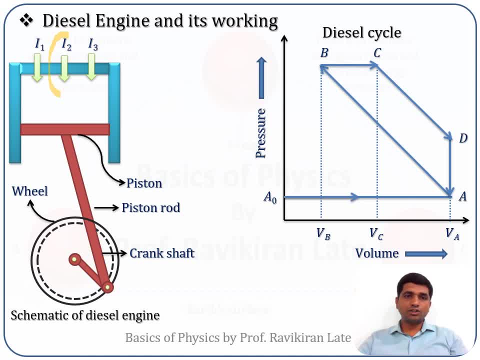 difference is there? in auto engine there were spark plug was provided, but in case of a diesel engine you don't need a spark plug. we'll be discussing that, why we spark plug is not required in this one during the multiple choice question sessions. the so diesel cycle- it is shown over here, which also consists of a six operations. the operation one: 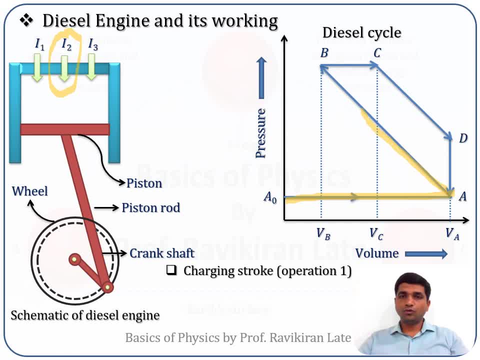 that is, a naught to a operation, two, from a naught to a daughters to a parleau, which is exponential, and then after that the next stage model is provided, and then after that, the next stage model is provided, and then after that the next a to b, operation 3 from b to c, operation 4 from c to d, operation 5 from d to a and the. finally, 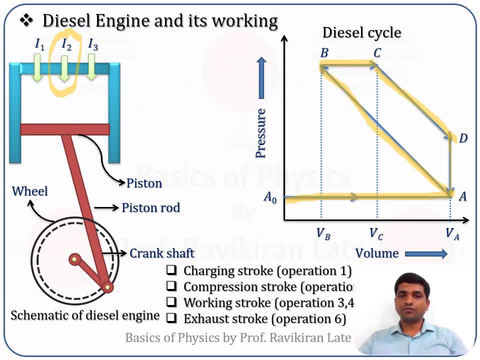 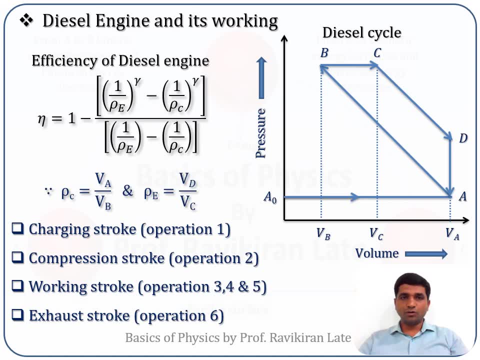 the exhaust operation. it will be there, which is from a to a naught now see all these operations we will discuss in the detail over here. in the first operation the fluid will be taken inside, or the gases or working substance it will be taken inside the chamber during the 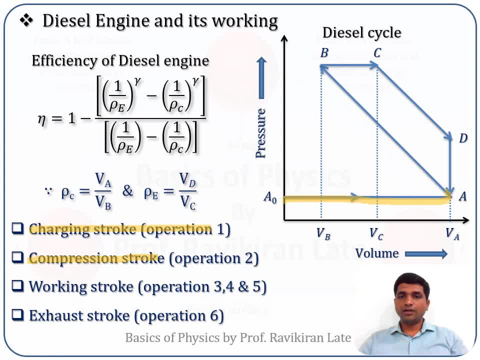 second phase, it is the compression stroke in which the volume of the fluid or the fuel which is there, it will be compressed, which is operation number three. in the third case, which is a working service stroke, there are three operations are there, from b to c, c to d and d to a, in which 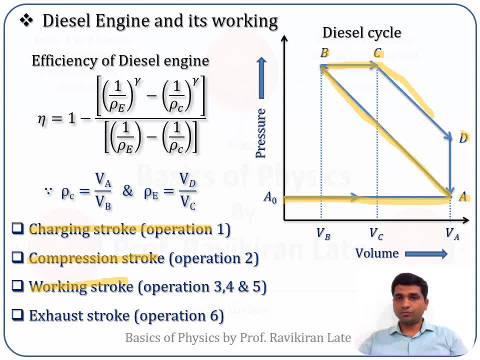 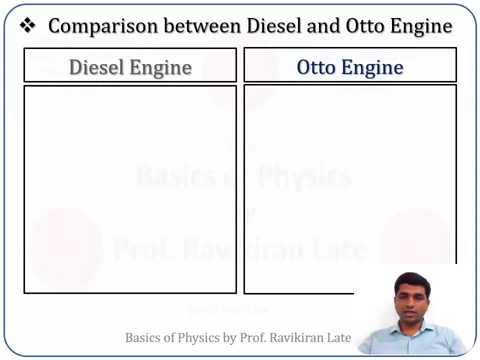 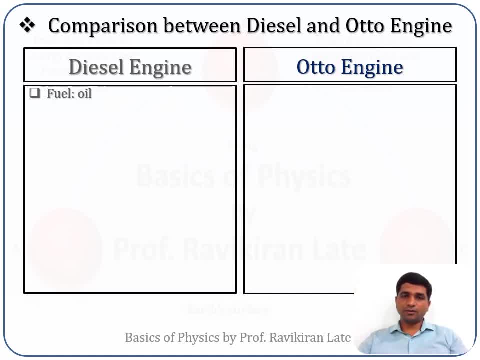 engine and the auto engine. now see, in case of a diesel engine, it is a oil which is used, as in case of a diesel engine, it is a oil which is used, as in fuel, where in auto engineer, its petrol or combustible gases are used for a fuel purpose. 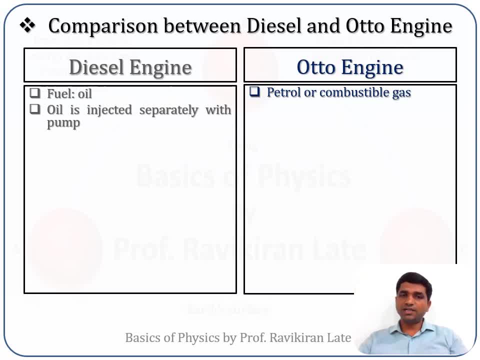 fuel. where in auto engineer its petrol or combustible gases are used for a fuel purpose �rally in diesel engine oil is injected separate with the help of pump, but in case of auto engine no pumps are required. petrol or air pressure and air. it is uh admitted directly as a mixture in this auto engine heat during an uh disaster occurs also. 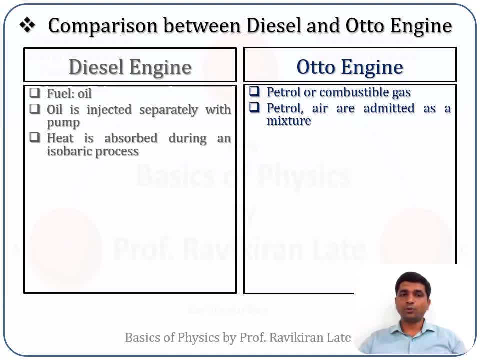 diesel engine, it is absorbed during an isobaric process. Remember this: during a diesel engine, heat is absorbed during an isobaric process, whereas heat is rejected during an isochoric process. In case of an auto engine, heat is absorbed during an isochoric process. 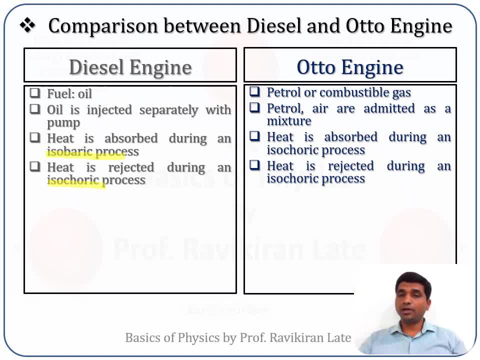 whereas heat is rejected also in during a isochoric process. we will see this in the cycle as well. while discussing the multiple choice questions next, adiabatic compression causes the ignition in case of a diesel engine, because we had seen no spark plug is used in case of a diesel engine, whereas in case of an auto engine, electric spark. 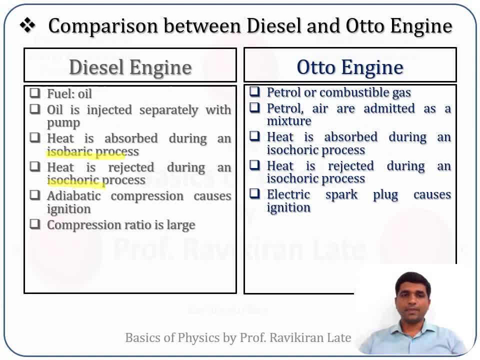 plug is used and which provides a ignition, in diesel engine the compression ratio is large, whereas in case of auto engine, the compression ratio is very small if you consider the danger of explosion. in case of diesel engine it has relatively lower, low danger of explosion, whereas in case of, as the combustible gases or petrol is used, so it has high risk of a. 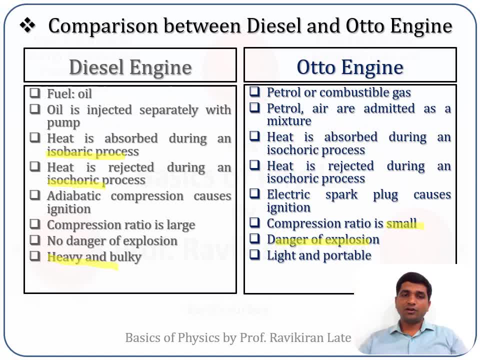 ignition, so it has high risk of a ignition, so it has high risk of a ignition, so it has high explosion. In case of a diesel engine, these types of engines are very heavy and bulky, They are not portable devices, Whereas the auto engines are little one or lighter in size and shape. 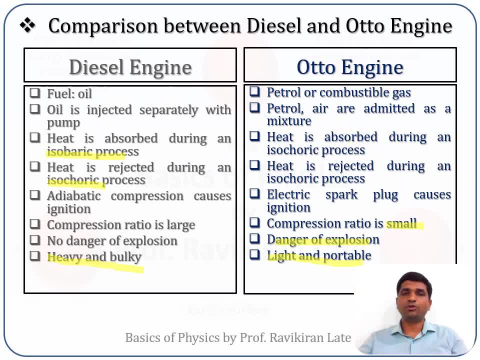 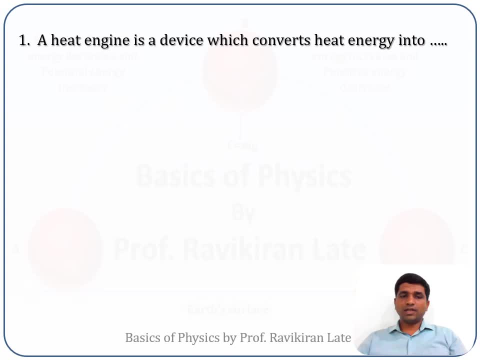 and they are portable, You can transport from one point to the another point. So, and if you consider from the efficiency point of view, diesel engine have a high efficiency as compared to the auto engine. Now, that was the theory which we wanted to discuss. Now we will discuss. 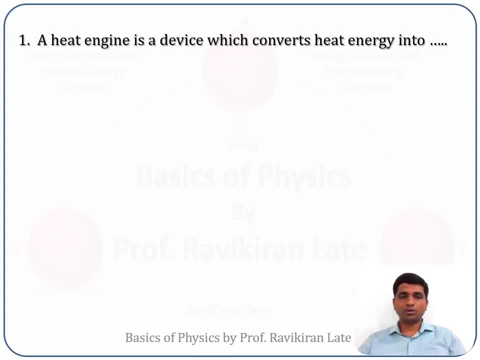 the some of the important multiple choice questions based on the theory which we have considered Now. first question is: a heat engine is a device which converts heat energy into option A- mechanical energy, option B- electrical energy, option C- sound energy, option D- chemical energy. Now, just in the during the 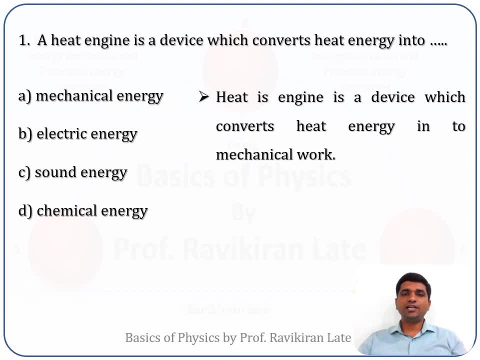 starting of this lecture only we had seen. heat engine is a device which converts heat energy into the mechanical work. So if you look into the option, it is the option A which suggests it is the mechanical energy. So heat engine is a device which converts heat energy into the 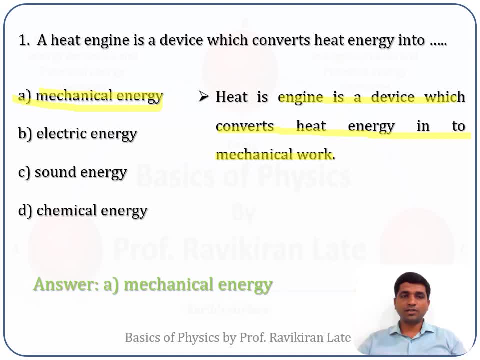 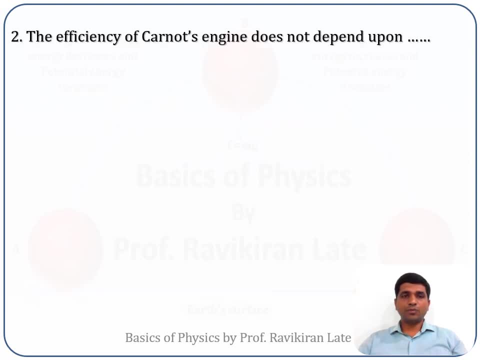 mechanical energy. So in this case the correct option is the option number A, mechanical energy. Next next multiple choice question is: the efficiency of Carnot engine does not depend upon option A- temperature of source. option B- temperature of sink, option C- nature of. 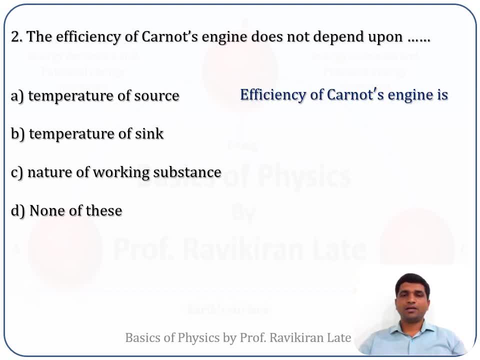 working substance. option D: none of these. Now see efficiency of a Carnot heat engine. it is given by the formula: eta is equal to T1 minus T2 upon T1, where T1 is the temperature of the source, which is given in the option number A, T2 is the temperature of the sink, which is given in the 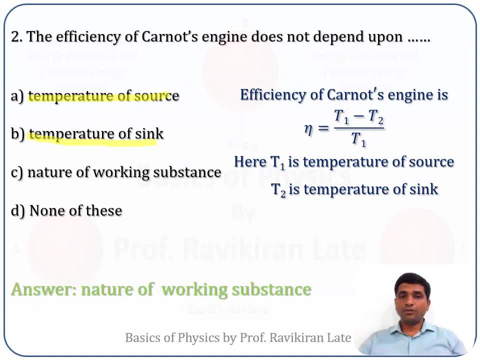 option number B. So if you consider the efficiency of a Carnot engine, it depends upon the T1, which is the temperature of the source, okay, and it depends upon the T2, which is the temperature of the sink. So in question, as it is asked, the efficiency of Carnot engine does not depend. 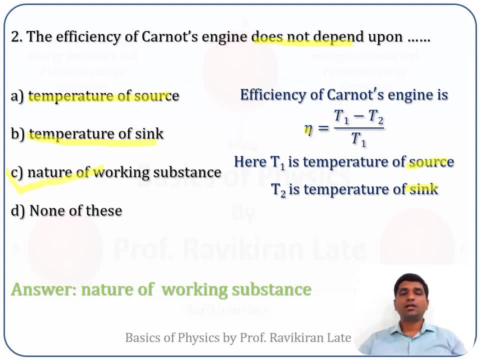 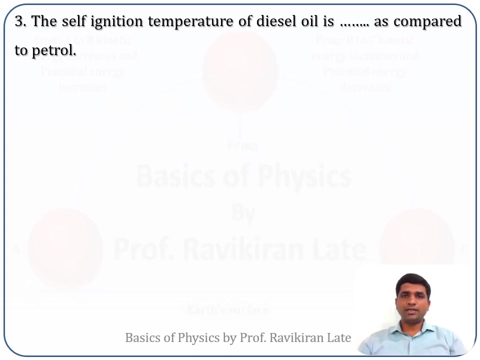 So it is the nature of the working substance on which the efficiency of a Carnot engine does not depend. So it is the option number C, nature of the working substance on which the efficiency of the Carnot engine does not depend. Now, next question is the self-ignition temperature of diesel oil is dash dash as compared to petrol. 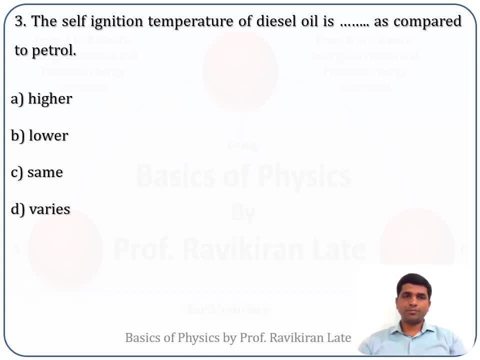 Options are given over here: higher, lower, same varies. Answer for this question is obviously lower. Now, first of all, we will try to understand what is self-ignition temperature is Self-ignition temperature is the lowest temperature at which a fuel will ignite. 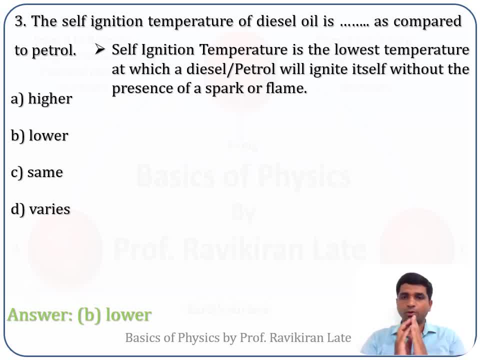 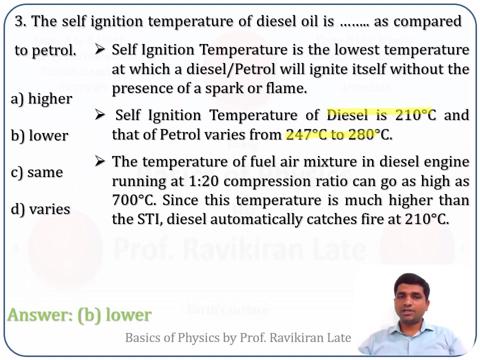 Ignite without providing a electrical spark. without providing an electric spark. In case of a diesel, the self-ignition temperature is 210 degree Celsius, Whereas in case of petrol, it varies from 47 to 280 degree Celsius. Now, temperature of fuel. air mixture in diesel engine running at 1 as to 20 compression ratio. 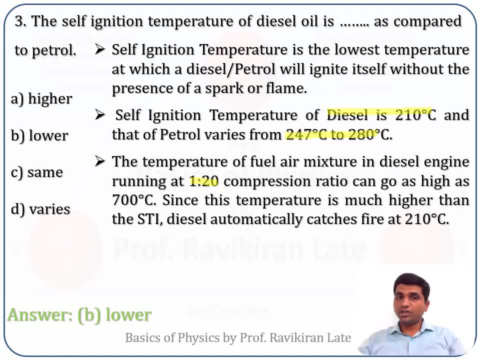 And this compression ratio can give a temperature of around 700 degree Celsius, As this temperature is much higher than the self-ignition temperature of the diesel, which is 210 degree Celsius. So due to that one, the diesel can catch fire easily. 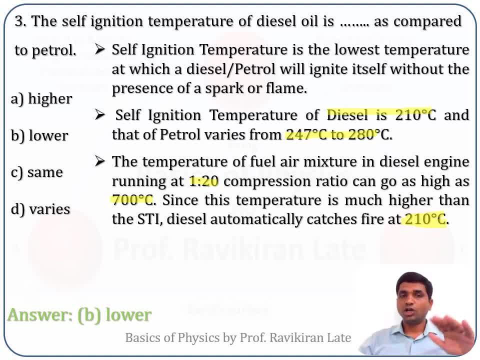 Or self-ignition temperature. This temperature, Due to the compression, the temperature of the mixture, it will be above self-ignition temperature. So due to that one, you don't require a spark plug in case of a diesel engine. 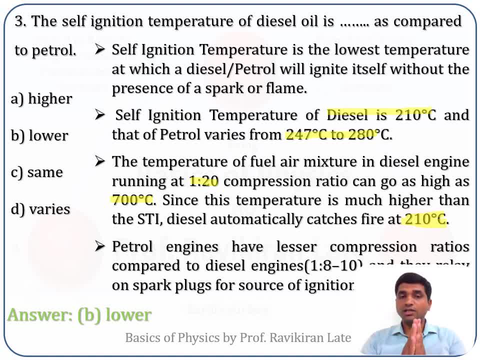 Whereas, on the contrary, in case of a petrol engine, you have a lesser compression ratio. The compression ratio is generally 1 as to 10 to 1 as to 8. And this does not provide that much amount of temperature, That much self-ignition temperature- okay for a petrol. 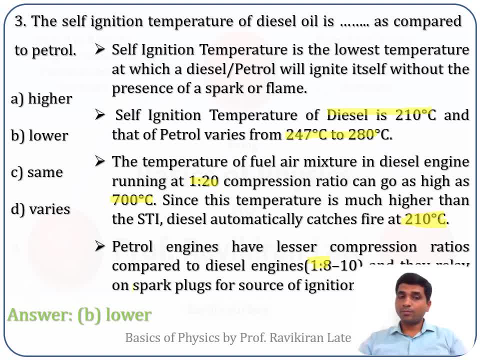 So, due to that reason, it is the spark plug which is used for the in case of an auto engine, or petrol engine for the purpose of ignition. Okay, So in this case, if you consider this question, the self-ignition temperature of the diesel oil is much lower than the petrol. 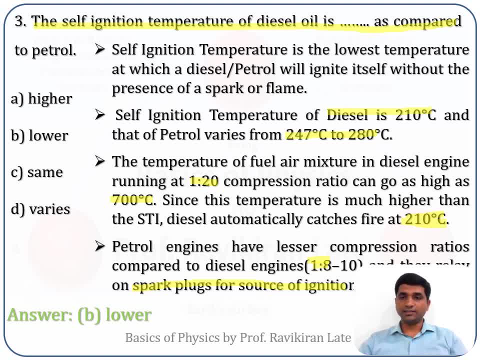 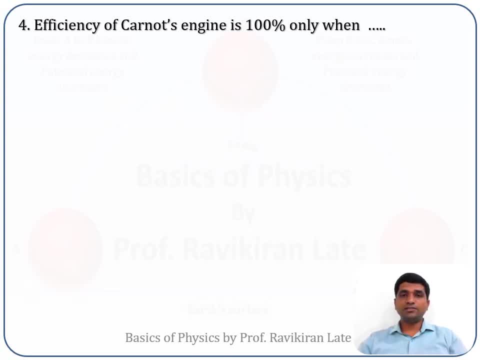 Okay, It is a 210 degree Celsius. Fourth and multiple choice question is: efficiency of Carnot engine is 100% only when option A: sink is at 100 degree Celsius, sink is at absolute zero, sink is at room temperature, sink is absent. 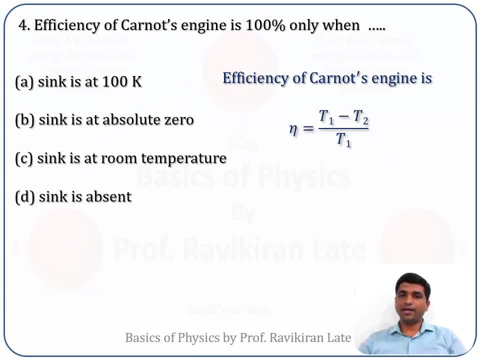 We know that efficiency of Carnot engine- it is given by eta A- is equal to T1 minus T2 divided by T1.. T1 minus T2 divided by T1.. Now what I will do? I will divide this T1, I will give this denominator to each of the numerator. 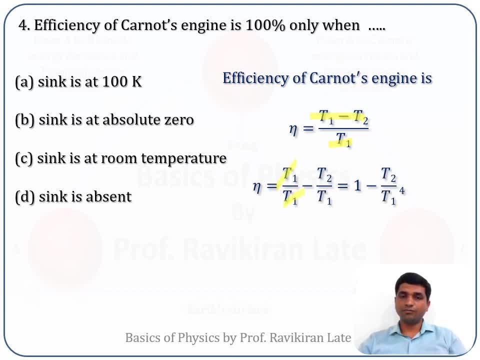 So if I do that one, this T1 can cancel with this T1. And so it will be 1 in this case. So it will be 1 minus T2 upon T1.. Now, if you consider, in this case we need to. it has been asked to us what is the condition when you will get a 100% efficiency. 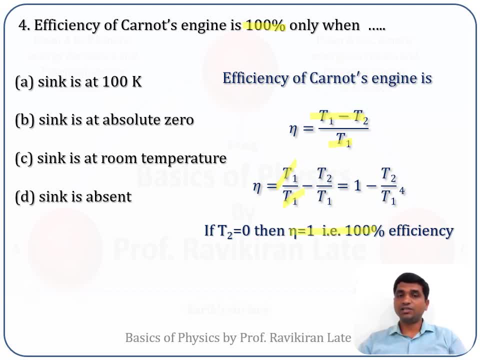 Okay, If we, if we need to have a 100% efficiency, then this second term has to be zero, And this can be possible only when this T2 will be zero. So that means it is T2 is the temperature of the sink. 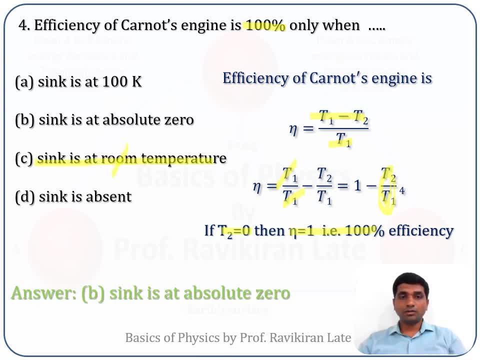 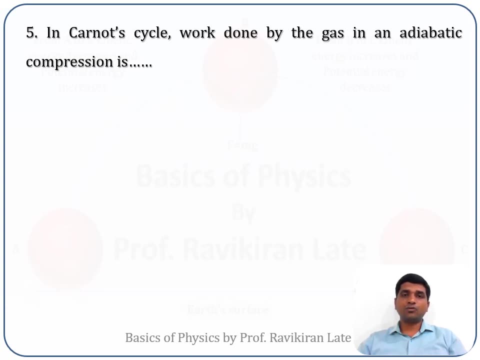 So temperature of the sink has to be. temperature of the sink has to be zero at absolute zero. So the correct answer for this question is the option number B. Next multiple choice question is: in Carnot cycle work done by the gas in adiabatic compression. these are the options which are given over here. 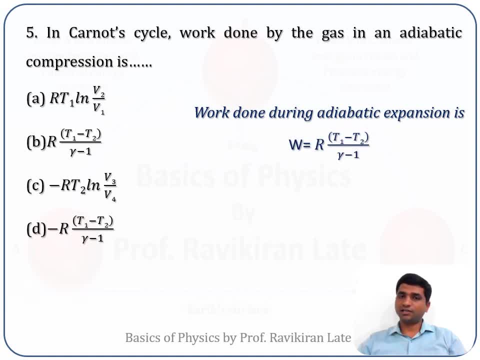 We know that work done during an adiabatic expansion is given by W is equal to R T1 minus T2 upon gamma minus 1.. As it is an adiabatic expansion, we need to find out a work done for an compression. 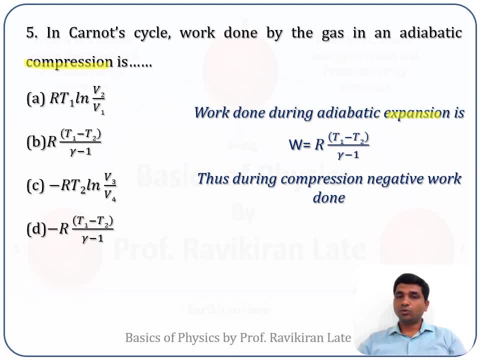 We know that during an compression process the work done is just opposite, That is, a negative Of the expansion. So in this case, if I do the give the negative sign to this one, So in this case, the work done during an adiabatic compression, it will be the option number D minus R, T1 minus T2, divided by gamma minus 1.. 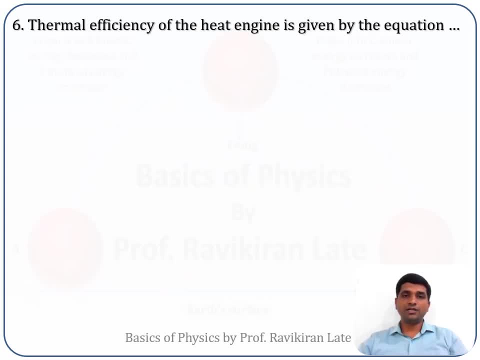 Sixth question is: thermal efficiency of the heat engine is given by the equation, option A: 1 minus Q2 by Q1.. Q2 by Q1.. Q1 by Q2 minus 1.. 1 minus Q1 by Q2.. 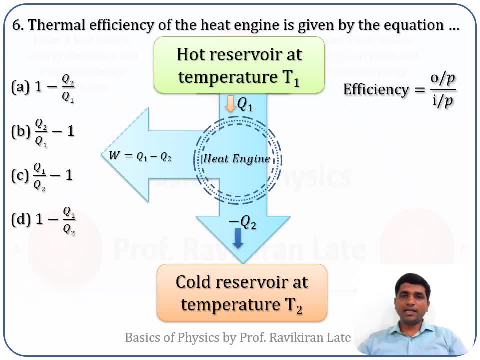 We know that a thermal efficiency of any engine it is nothing but the output we are getting per unit input. Okay, So in this case we know that any kind of a heat engine it gives it takes some amount of heat from the heat reservoir. 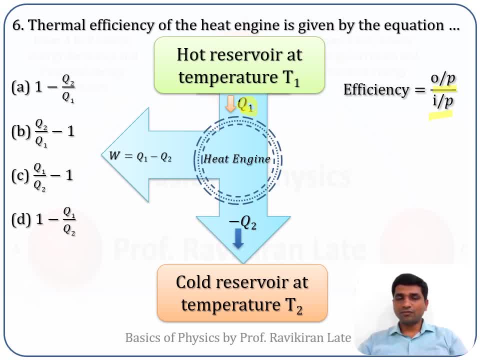 So let us say Q1 is the amount of heat which is taken from the heat reservoir And minus Q2 is the amount of heat which is given to the cold reservoir. So in this case the net heat which is converted into work it is Q1 minus Q2.. 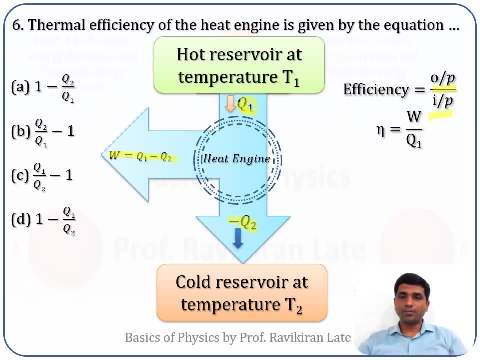 So you can write down the efficiency, that is, work obtained, divided by the amount of heat provided. That is, W upon Q1.. But W is nothing but the Q1 minus Q2.. So if I substitute it in this one, now what I can do, I can divide this Q1 to each of these. 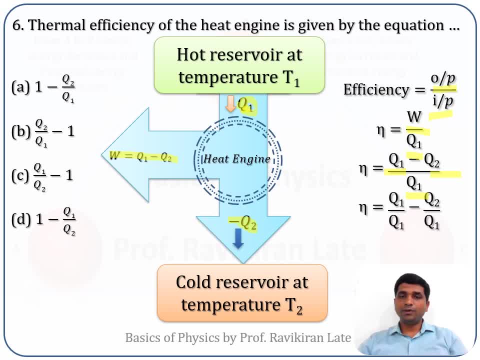 This term Q1 and Q2.. If I do this, it will be Q1 divided by Q1 and this Q2 divided by Q1. This Q1, Q1 will get cancelled each other, So you will get 1 minus Q2 by Q1. 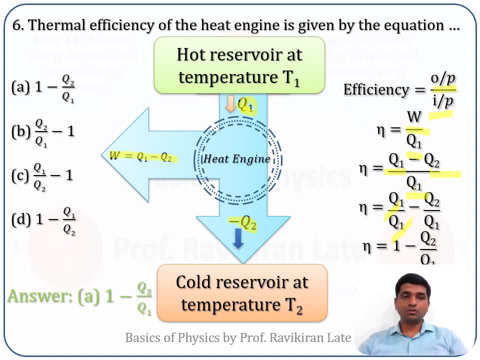 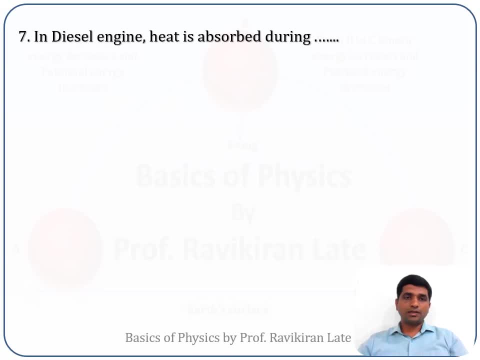 So that is nothing but the option number D. in this case, The correct answer for this question is option number D. Next question is: in diesel engine heat is absorbed during option A- isothermic, Option B- adiabatic process. 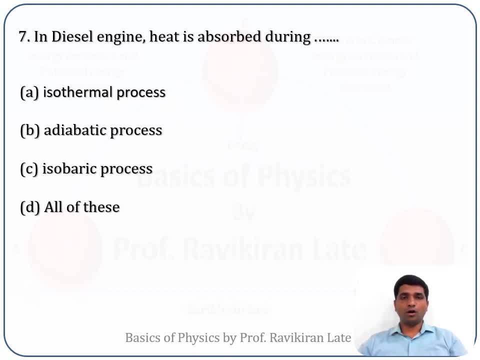 Option C: isoparic process. Option D: all of these Now in our theory part, we had seen a diesel engine. it has this cycle. If you consider, in case of a diesel engine, heat is absorbed during this process. 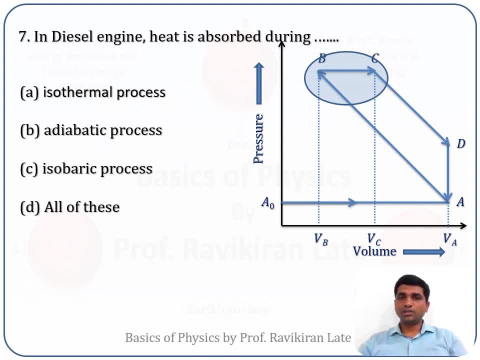 During the curve, PC heat is absorbed. If you consider from B to C, from B to C, that is WB2C, The volume of the system remains. volume of the system increases from this point to this point, But the pressure at this point, these two points- remains same. at this point. 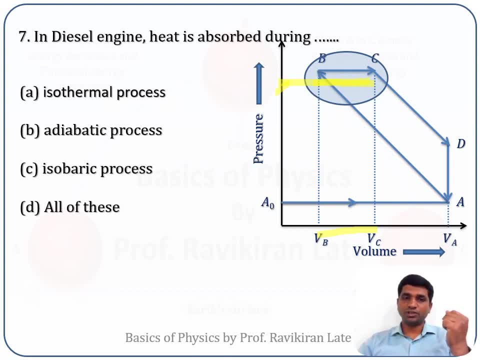 So it is. the pressure is constant during this process And we know that the pressure, if the process during which pressure is constant, such a kind of process is called as a isobaric process. So the correct answer for this question is the isobaric process. option number c. next question: in petrol engine in. 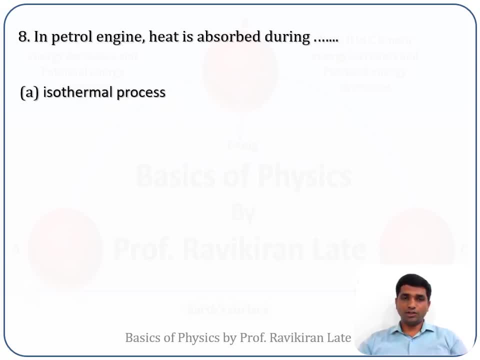 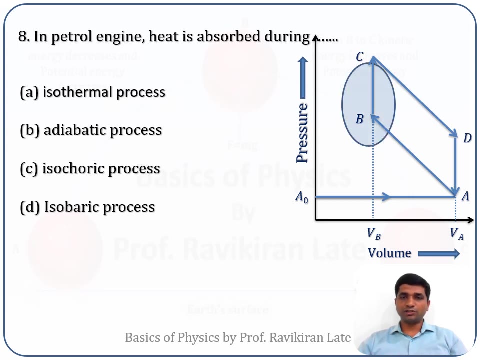 petrol engine heat is absorbed during isothermal process, adiabatic process, isobaric process. sorry, isobaric process and isobaric process. now we know that, in case of an petrol engine, the heat is absorbed during this process b, c and if you consider, during this b c. 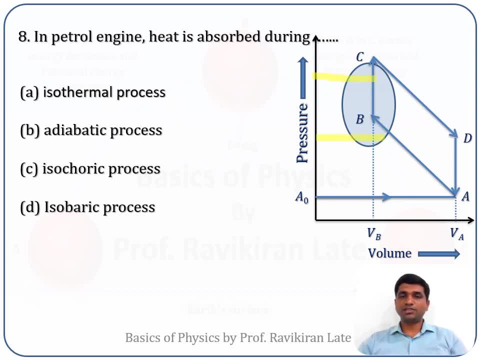 b and c. the pressure of the system remains constant, but it is the volume which is remaining constant at the point b. so, if you consider, the pressure is changing but volume is remaining constant, so the process during which volume remains constant, we know that that process is constant. 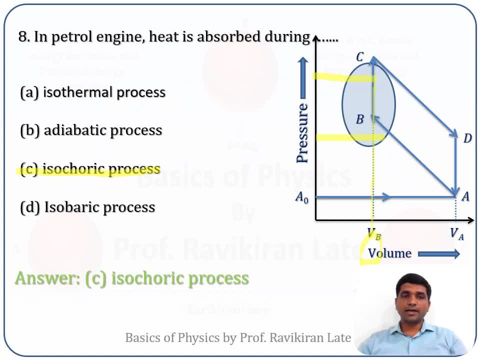 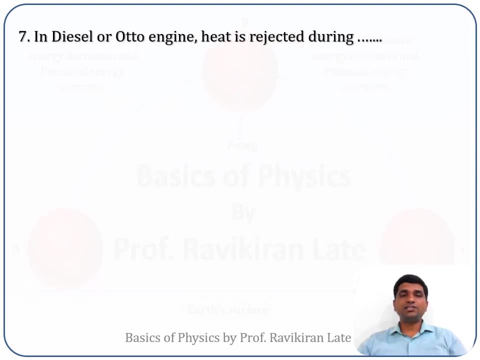 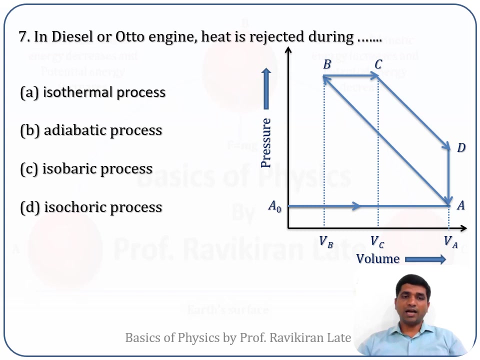 as a isochoric process. so the correct answer for this question is that is the process, isochoric process- during which petrol heat engine absorbs a heat. option number c. next question is: in diesel engine or auto engine heat is rejected during isothermal process, adiabatic process, isochoric? 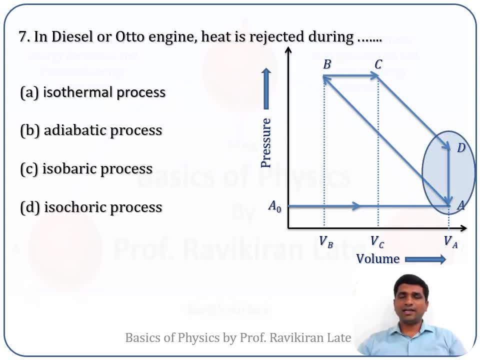 process, isobaric process. we know that in case of an auto engine or a diesel engine, heat is rejected to the system during the curve da and during this process, if you see, it is the volume which is remaining constant. in this case, pressure is changing from this point to this point, but volume. 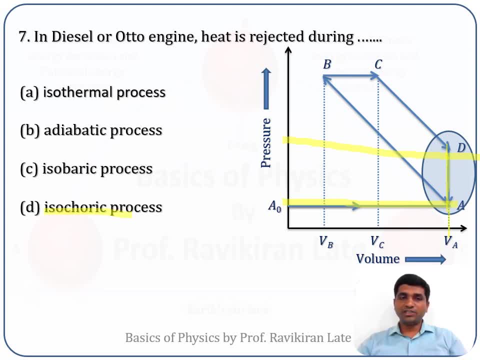 remains constant and we know, all of us know, that if the pressure is remaining constant, if pressure is remaining constant- sorry, if volume is remaining constant, then it is the isochoric process. so the correct answer for this question is isochoric process. last three questions which we have discussed, it tells us that 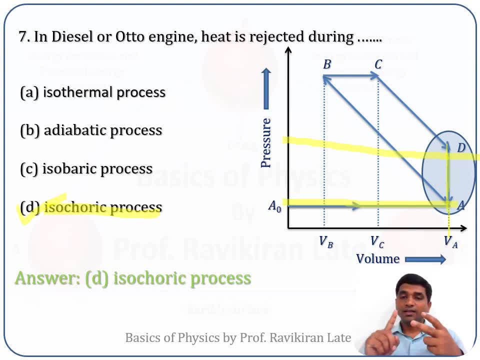 in case of an auto engine or a diesel engine, the heat is absorbed during the different processes, but in case of an auto engine or a diesel engine, the heat is rejected during a same process and that is nothing but the isochoric process that you have to remember that. what question is exactly asked during the exam? 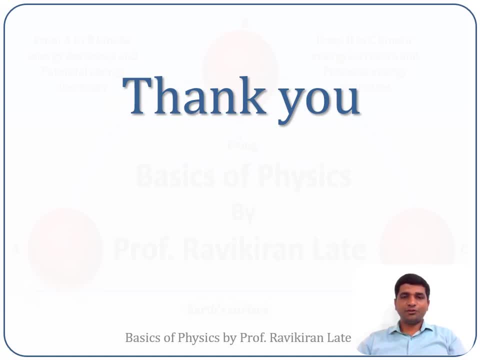 that's it for the today's session. i thank you all, students, for attending the sessions. i request all of you to please like and comment in the videos and, if you have not subscribed our channel, please, i request all of you to please subscribe and please share this content with your friends from. 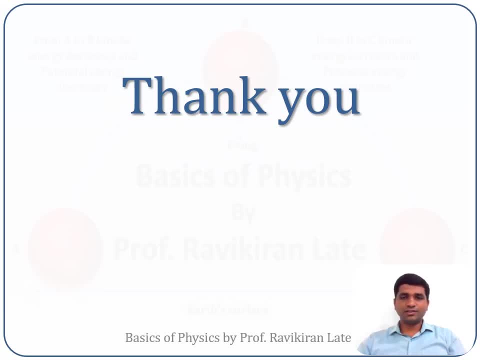 the other colleges. okay, that's it for the today's session. we'll stop here for the today's lecture. thank you. 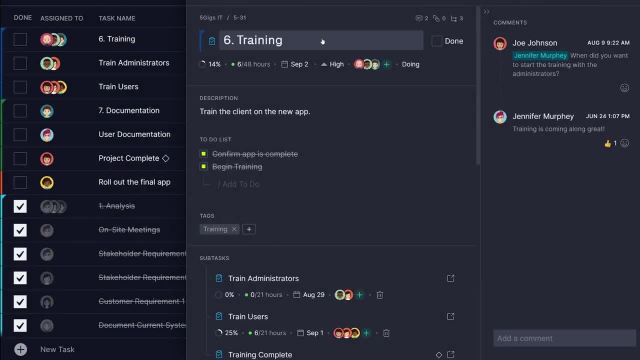 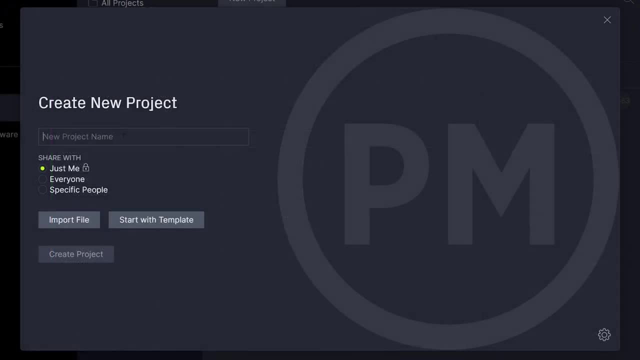 Welcome to Project Manager, your new platform to plan, monitor, collaborate and report on your projects. We're excited to get you going on your project management journey. Let's start at the beginning, creating your first project. It's important to get your project started off on the right foot. 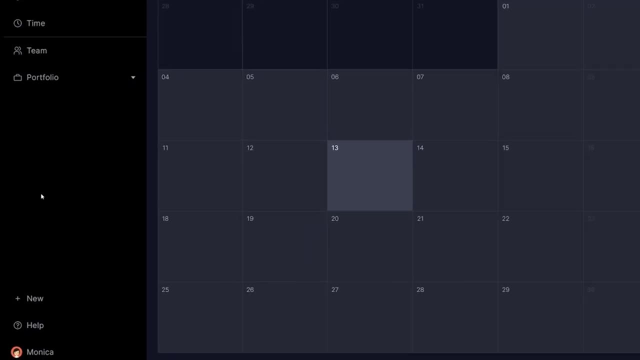 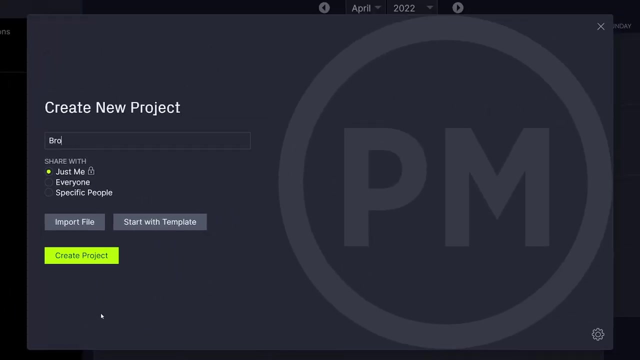 which is why Project Manager makes the process simple. To create a new project, simply click the plus icon and select Project. Give your project a descriptive name. then decide who you want to have access to it. To add additional information, click the cog in the bottom right. 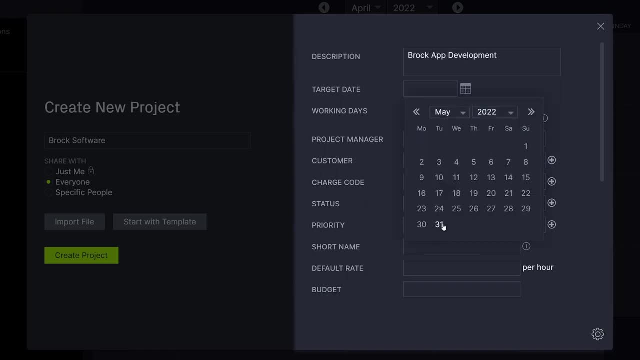 corner. Here you can set your project: working days, customer budget, priority and more. You'll also see multiple options for starting your project. You can import a file which looks like this: You can also import a file that looks like this: You can import a file that looks: